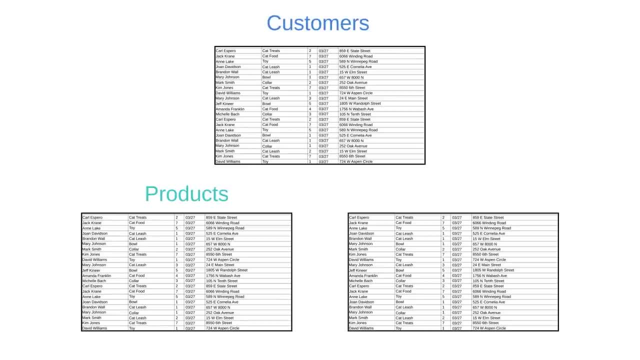 information into all of your customers, and then a separate table that lists out all your products and then another table that records each of your orders. This separates the data you're pulling in a much more efficient way. So here's what your customer table might look like. 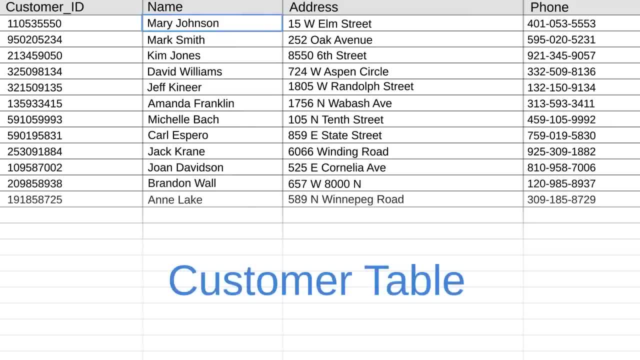 You can see we've got Mary again, but now she won't be repeated into several different rows. Any change to her address, contact info or even name can be updated in this one consolidated place. The product table would have all your cat accessory inventory as you add or remove items. 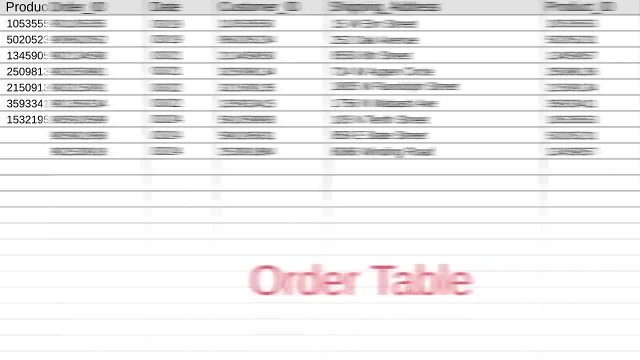 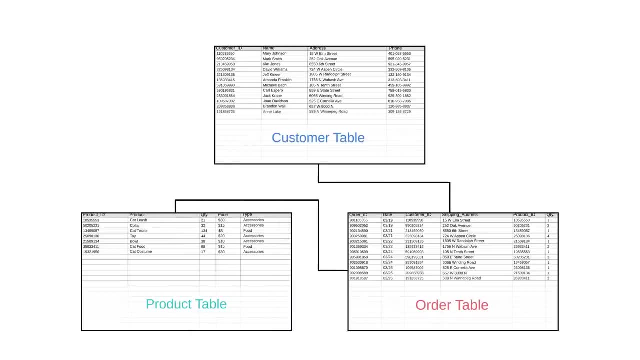 this would be the one place where you'd make those changes and orders, would keep track of every single sale you make. Now these tables, although separate, have connections to one another, and it's these connections that form the database. Let's dive in and take a closer look to see what 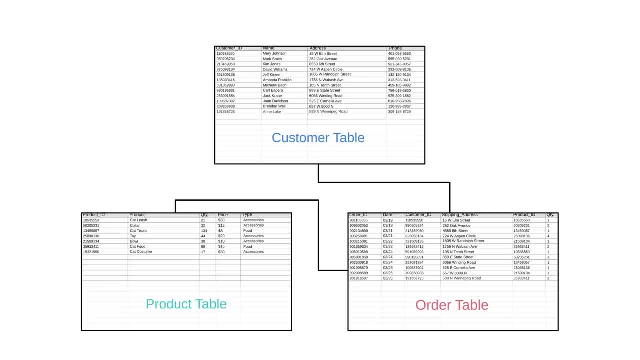 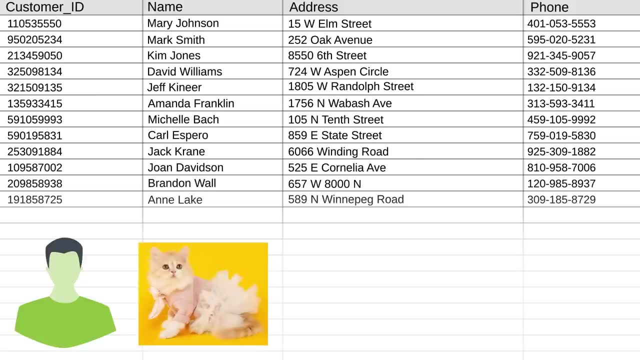 these interactions look like. We'll start in the customer table. Let's say someone goes to our online store and makes a purchase. It's a guy named Ronald and he's in the market for a cat costume and buys one from our store. When he checked out, he entered all his contact info. 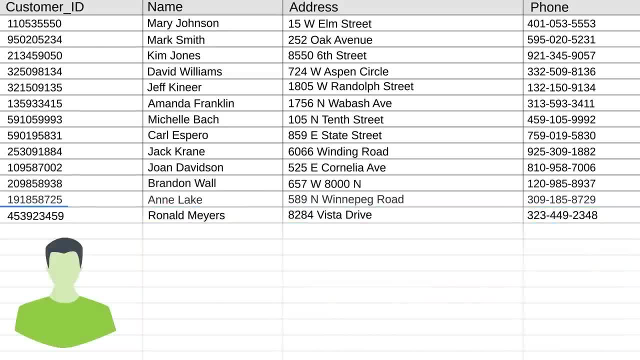 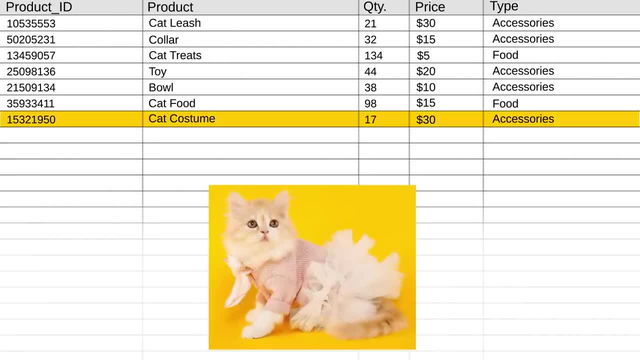 and we've recorded it and we've added it to our online store. So now we can see that we've got this customer table and assigned him a customer ID. Let's move over to the product table. This lists all our inventory and here's the cat costume he wanted. We keep track of it with a few fields. 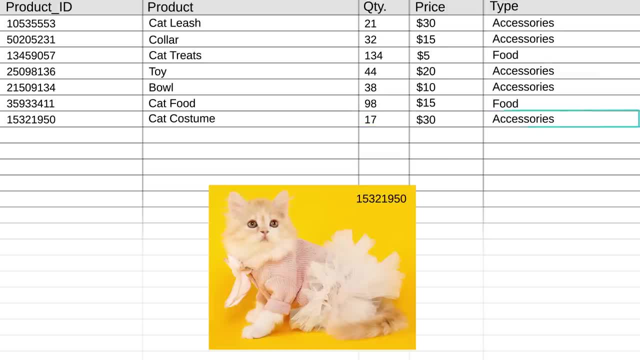 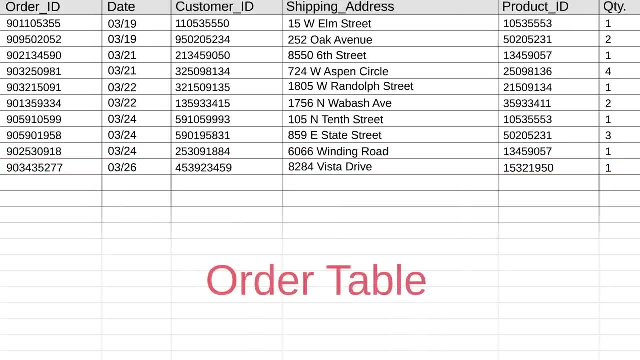 here like product ID, quantity in stock and product type. And then when Ronald actually ordered the cat costume, we record that specific purchase information in the order table. Here you can see we pulled in the customer ID from the customer table so we know it's Ronald. We also 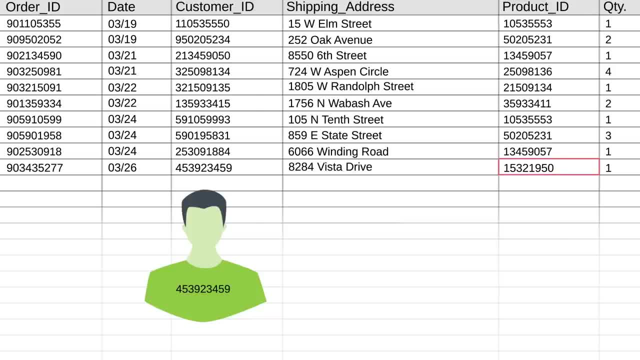 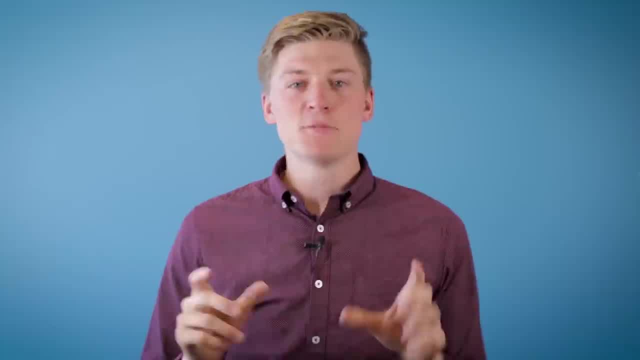 pulled in the product ID from the product table, so we know that he purchased this cat costume, And there's other data in here that tells us about the date of the sale, shipping address, quantity, etc. It's pretty obvious that this system we're using now is far more organized. 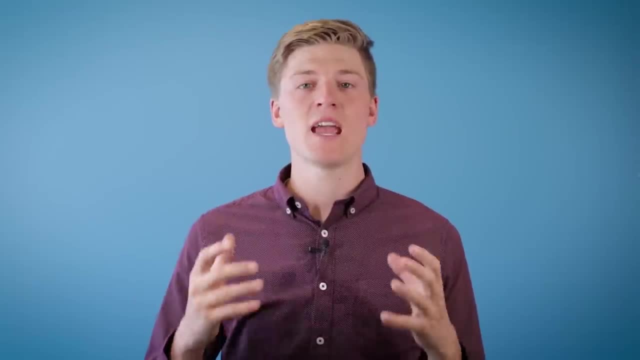 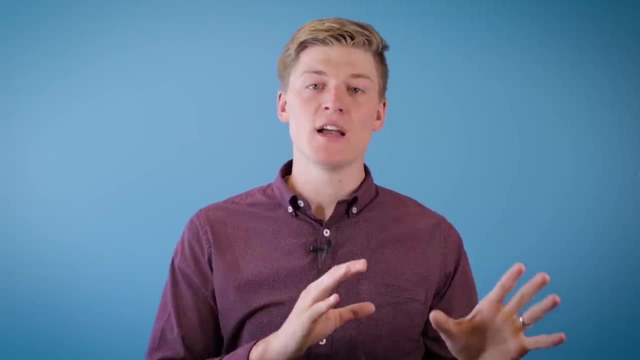 than our single-spice sheet from earlier, Not to mention it's far more robust in handling large amounts of data and information. But database management systems typically aren't very good at visualizing the tables and connections within a database. It's all in the programming language. 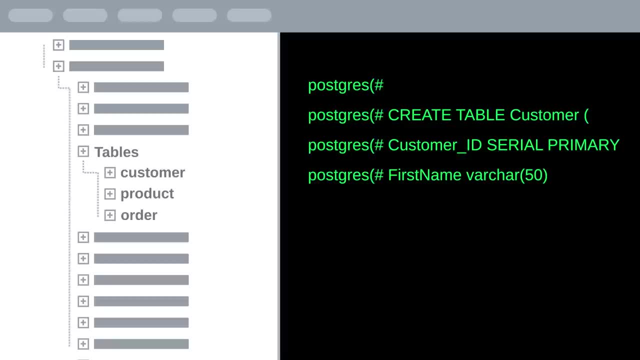 and it's hard to see where the connections are. So we're going to take a look at the programming language and it's hard to see where the connections are and where improvements can be made. That's where entity-relationship diagrams come in. It's a visual way of looking. 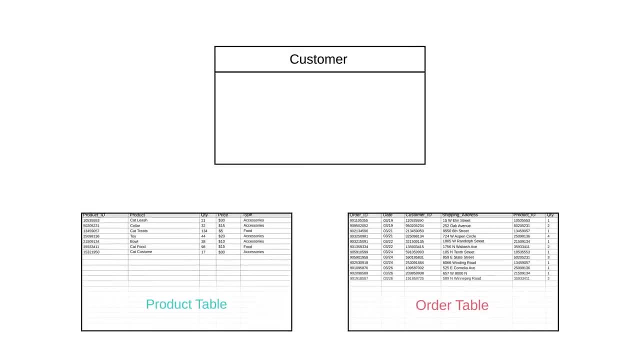 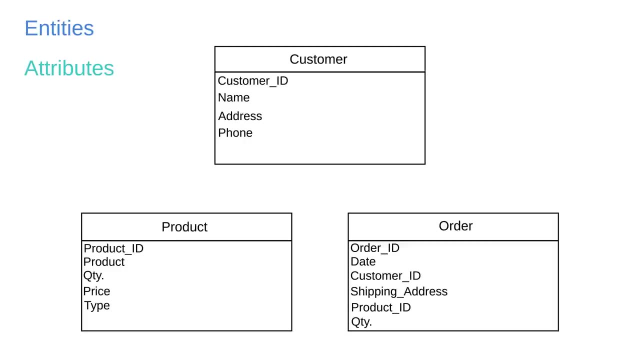 at your database structure. Each table translates into an entity And your column categories like customer name, address, purchase date, etc. are listed as attributes in their respective entity. Finally, the programmed connections between your tables, like how Ronald's order. 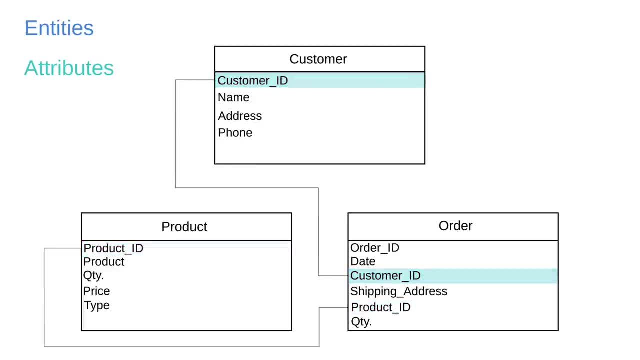 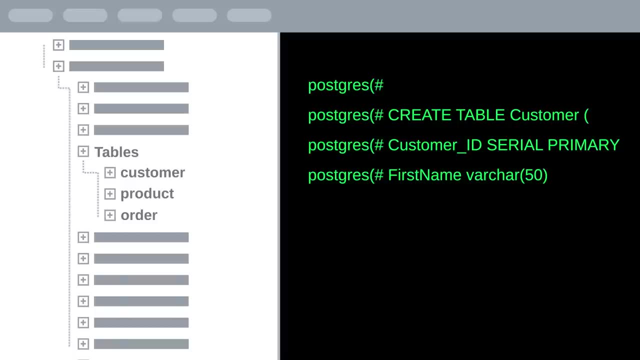 referenced a specific product ID and his customer ID. those are visualized through relationship lines. So imagine if your database was far more fleshed out than our simple example, like if you had separate tables for shipping address, billing addresses, credit card shipping info, etc. Trying to make sense of a large database. 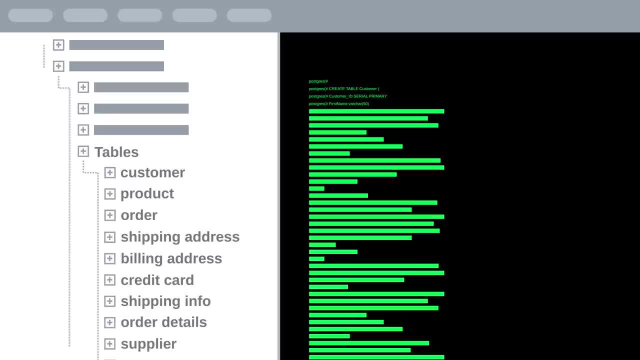 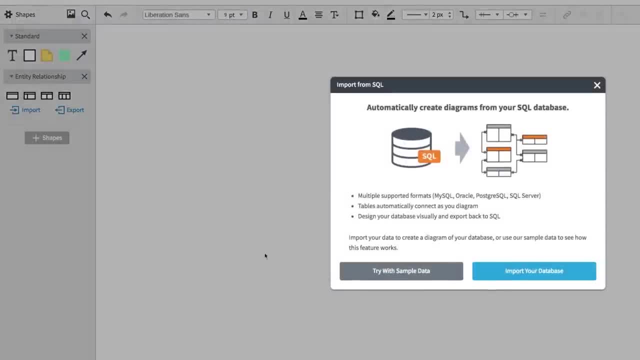 when you're in the database can be very taxing. It's much easier to visualize it through an ERD And that's a super-fast process with Lucidchart's ERD import tool. Just run a query of your database and Lucidchart automatically imports the tables that you can then drag out. 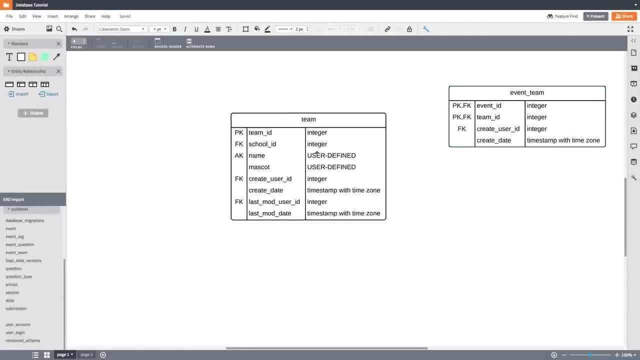 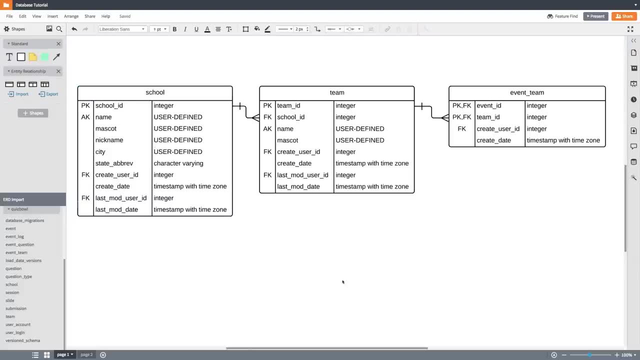 as entity shapes And the relationships between entities automatically connect as well. So you quickly create a visual representation of your database and then it's so much easier to spot database errors. you can see where you're getting duplicate data and it's way easier to onboard someone who's new to your database. They can look at an. 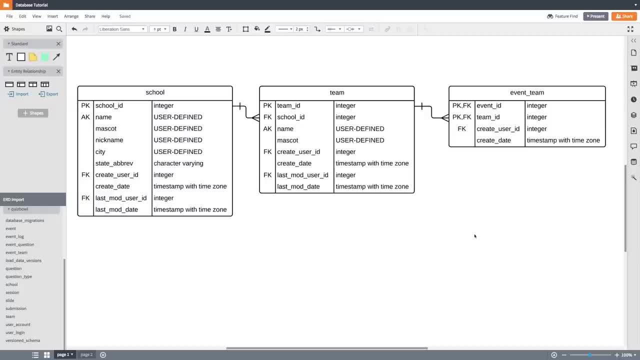 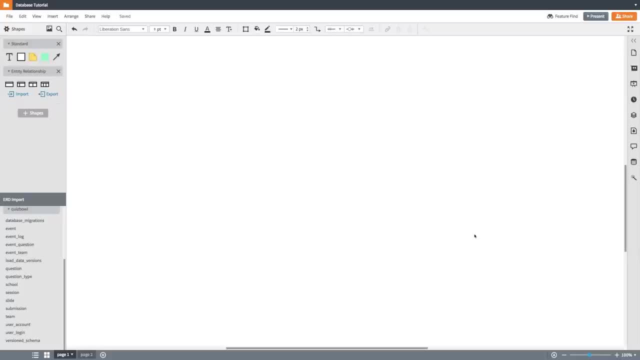 ERD and see how the whole thing works. On the flip side, let's say you don't have an existing database. You're starting from scratch and want to build one. Well, ERD is a great tool for concepting. You've got an idea for how your database is going to. 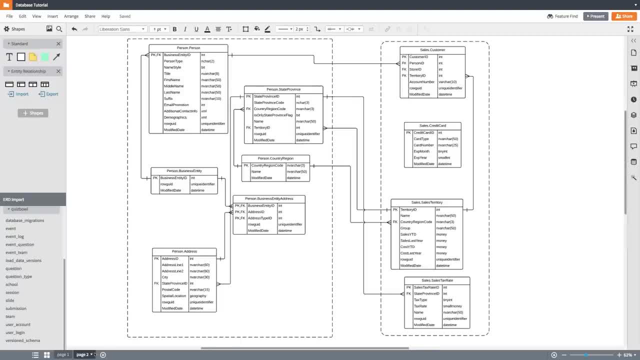 work and you flesh it all out in a diagram, And the awesome thing is that when you're done, concepting the diagram is going to be a little bit more complex, So you can see that the diagram itself can be translated into the code that forms the actual database. 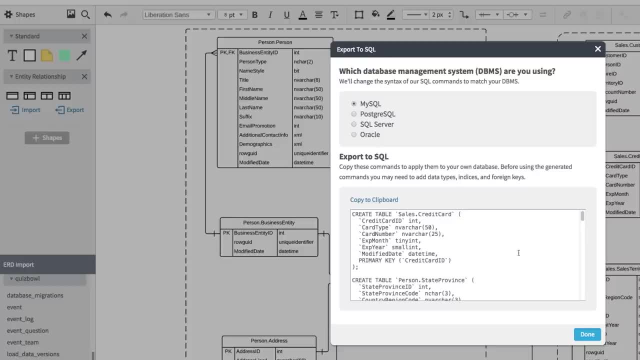 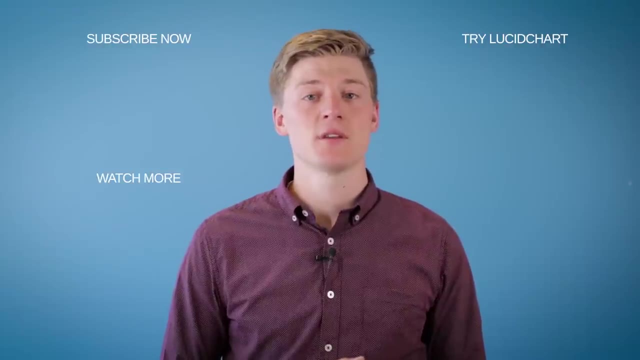 You don't have to manually recreate your concept in database form. The entities automatically transform into tables, the attributes to columns in those tables and your relationships get translated into coded connections. Hopefully this gives you a bit more context as to why we use databases and how they relate to entity relationship diagrams To learn. 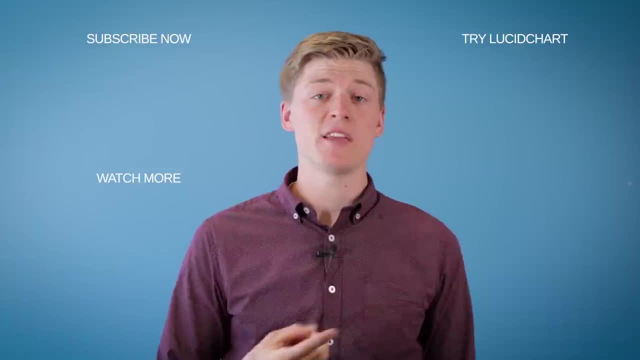 more about entity relationship diagrams in our other tutorials, like primary keys, foreign keys, attributes and cardinality- click here. Click here to start creating your own ERD diagrams today.